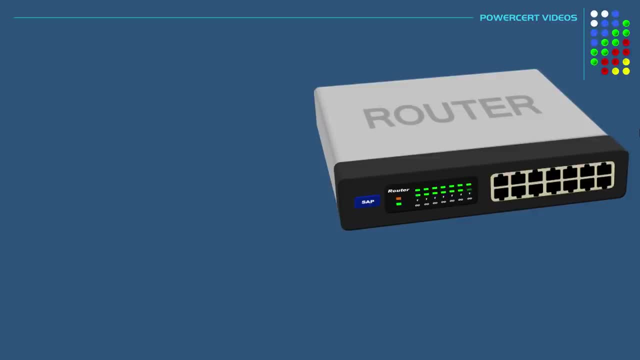 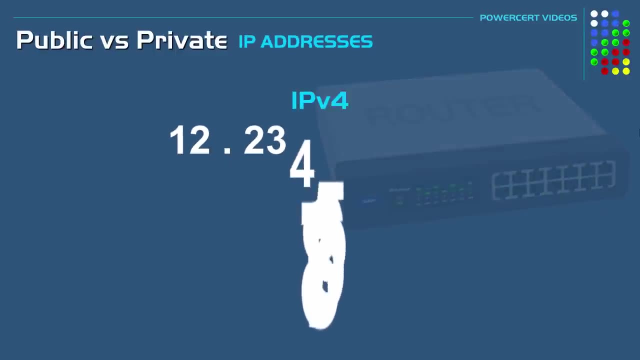 Hello everyone, in this video we're going to be talking about the difference between public and private IP addresses And, to be specific, I'm going to be talking about IP version 4 addresses. So the first thing we have to know is: what is an IP address? Well, an IP address is a numeric. 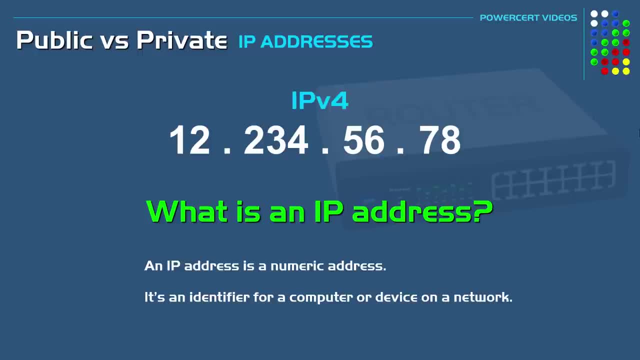 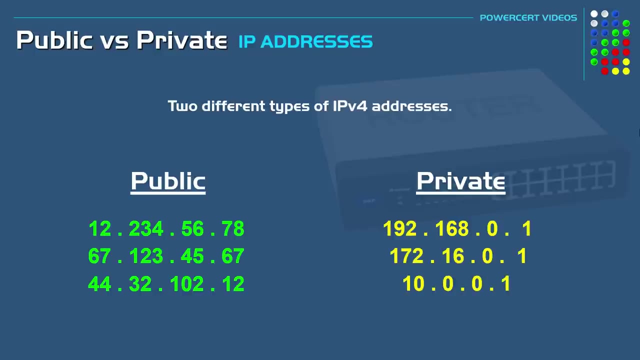 address. It's an identifier for a computer or device on a network. Every device has to have an IP address for communication purposes, And there are two different types of IP addresses: There's public and private. So what are the differences between the two? So let's first 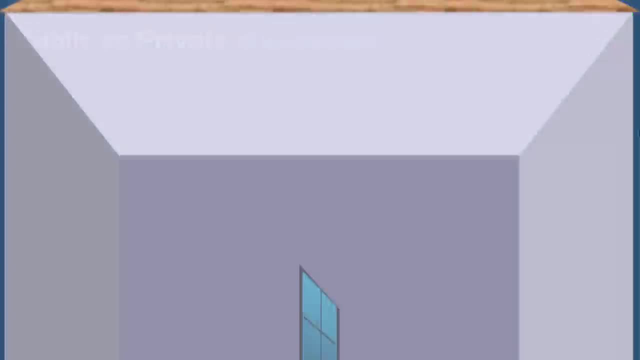 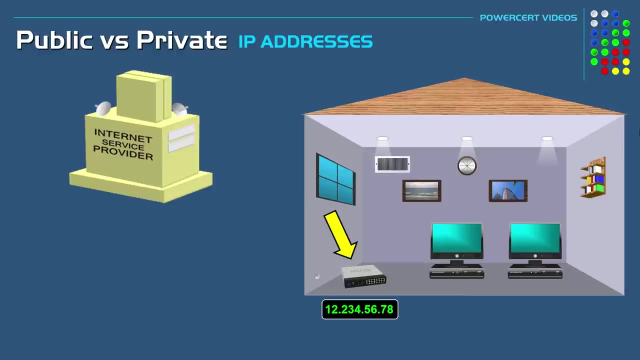 talk about public IP addresses. Now, when you order internet service from an internet service provider, they are going to assign your modem or your router in your home or business a public IP address. This public IP address is registered on the internet. It's what gives you. 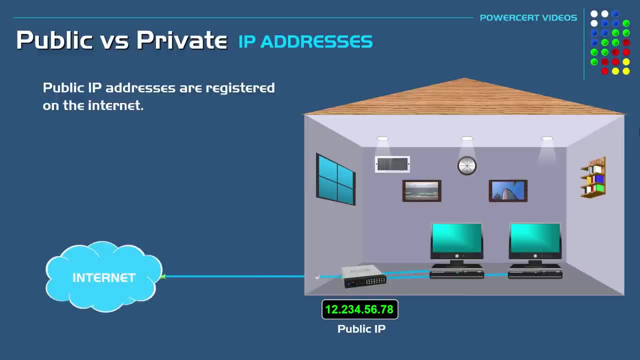 advertising information. to answer your questions or get tips for hitting ak mobile, You can click to the world wide web. So if you don't have a public IP, you cannot access the internet. Public IP addresses are also unique. There are no duplicates anywhere in the world of public. 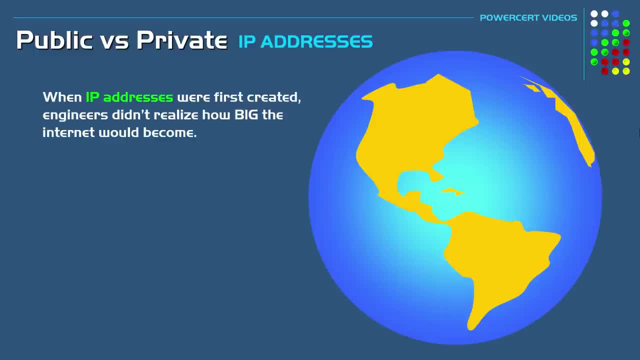 IP addresses. Now, when IP addresses were created, engineers didn't realize how big the internet would become, Because, even though there are over 4 billion IP version 4 addresses available, the engineers thought that this would be enough, But they were obviously wrong, because of the 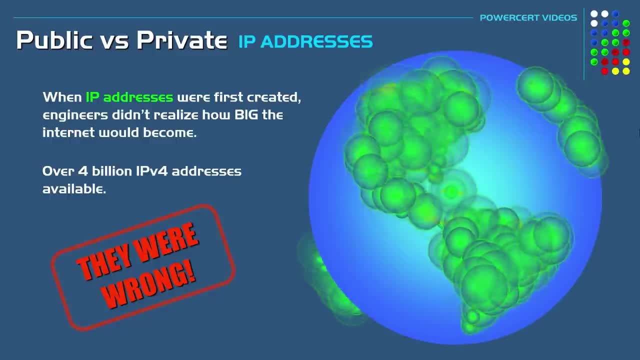 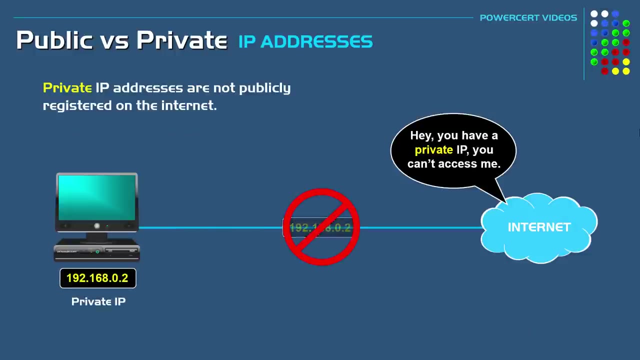 explosive growth of the internet. So in order to prevent a shortage of public IP version 4 addresses, engineers developed private IP addresses. Now, private IP addresses are not publicly registered on the internet, So you can't access the internet using a private IP address. 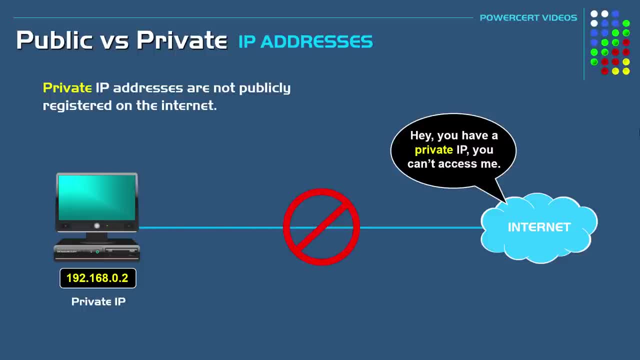 However, if your device does have a private IP address, it still has access to the internet. So if your device does have a private IP address address and you want to access the internet, your private IP has to be converted into a public IP address before you can access the internet. And this is because private IP addresses are only 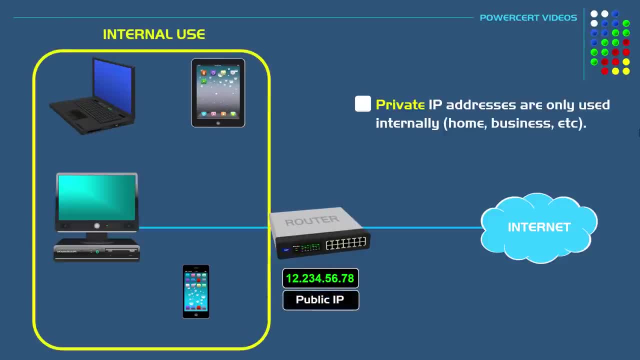 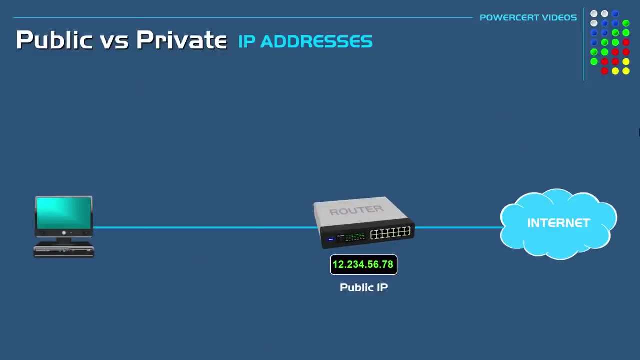 used internally, such as inside a home or a business. They are not used out on the public internet, And a service that's inside your router called DHCP, is what assigns your internal devices a private IP. So, as an example, most homes and businesses are not going to have just one device. 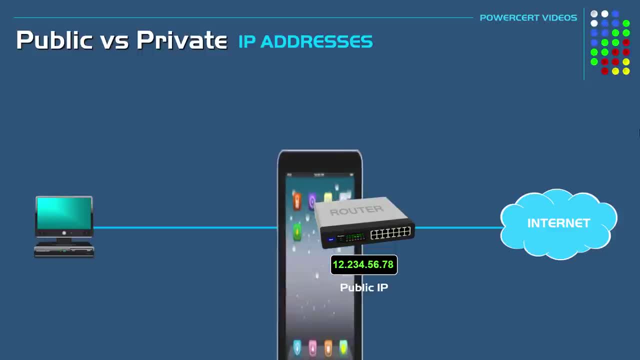 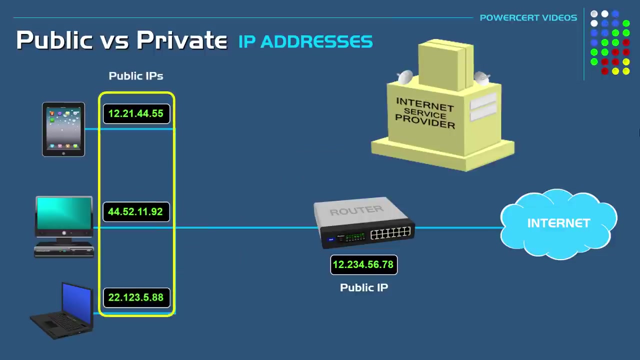 that needs access to the internet. Chances are they're going to have multiple devices that need internet access, So all of those devices need a public IP address if they want to access the internet. Now you could contact your ISP and ask them for these additional IP addresses for all of. 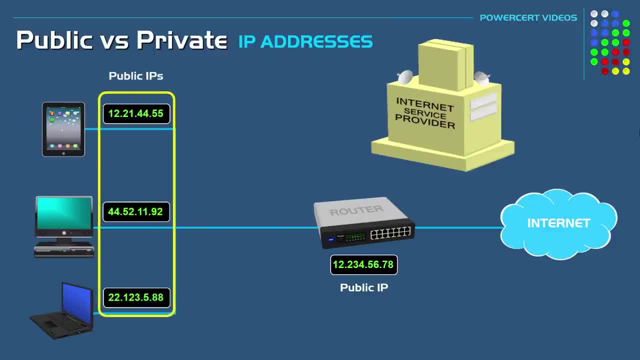 your devices, but that's going to be more expensive, unnecessary and more expensive than your internal IP address. If you want to access the internet, you need to have a public IP address. Now you could contact your ISP and ask them for these additional IP addresses for all of your devices. 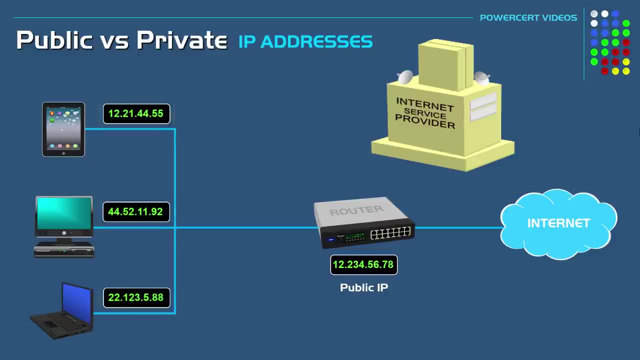 and, more importantly, it'll be a waste of public IP addresses. And let's face it: if every device in the world had their own public IP address, we would have run out of public IP addresses already. So what we can do instead is we can have the router assign the devices inside. 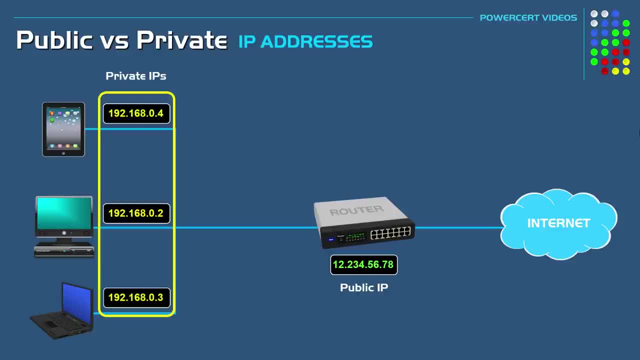 our home or business private IP addresses And when these devices need to access the internet, their private IP address will be translated to the one public IP address that we have been given, And the service that translates this is called NAT or Network Address. 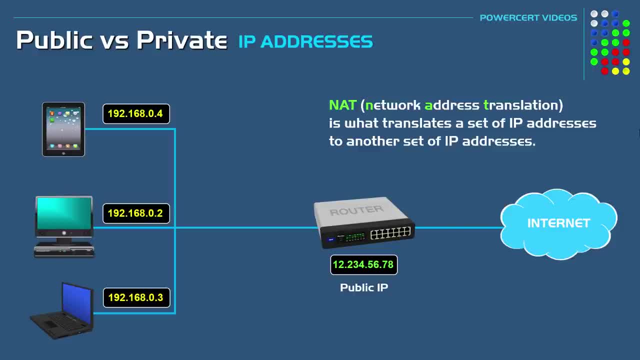 Translation, And it's a service that's built into our router, So not only does it translate private to public, but it also translates public to private, Because if a computer on the internet wants to communicate with a computer on this private network, the public IP address needs. 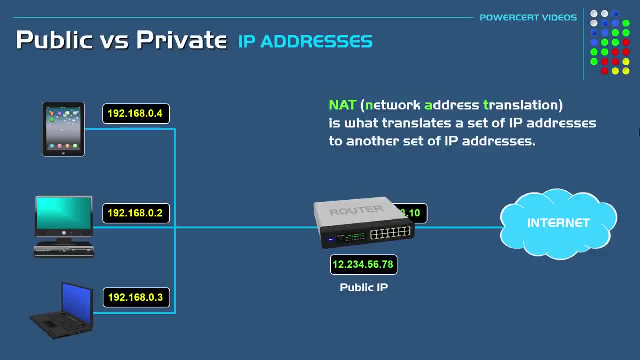 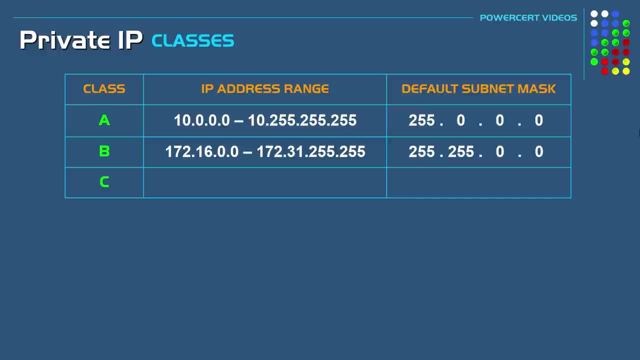 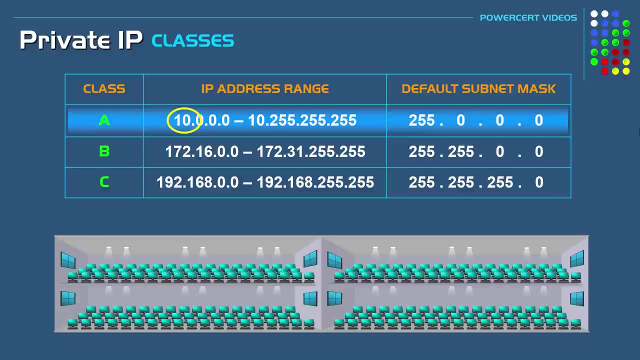 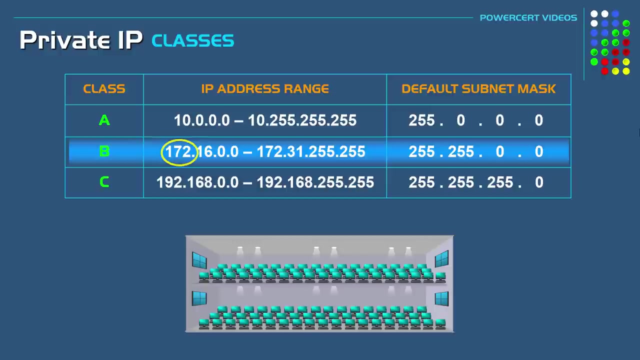 to be translated by NAT to the private IP address for that computer. Now private IP addresses have three different classes and these classes have different ranges. So a class A private IP starts with the number 10.. This class is typically used for large organizations. Class B starts with 172.. This is typically used in medium-sized organizations And 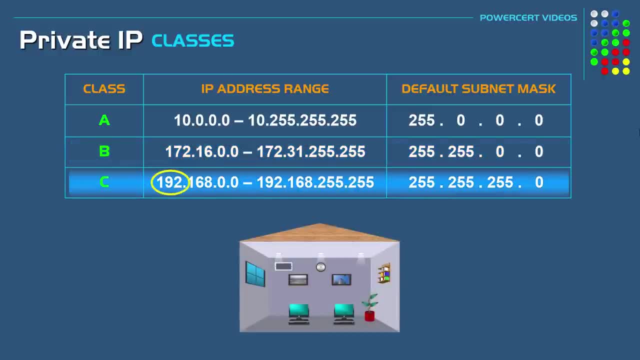 class C will start with 192. This is used in small organizations or homes. Class C is the most popular range of private IP addresses And class C is typically used in small organizations or homes, So don't be surprised if you happen to check your IP addresses on your devices in your home. 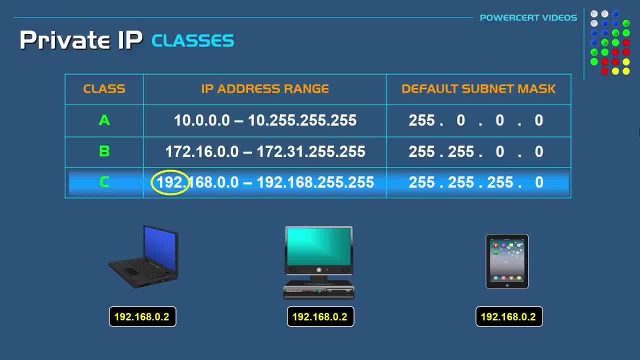 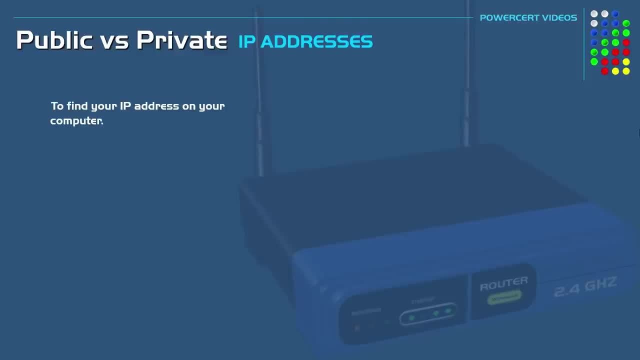 if you see them starting with 192.168. Because, like I said, it's the class that's mostly used. Now, if you want to find out what your IP address is, this is how you do it. If you're using a Windows computer, you just open up a command prompt and type: 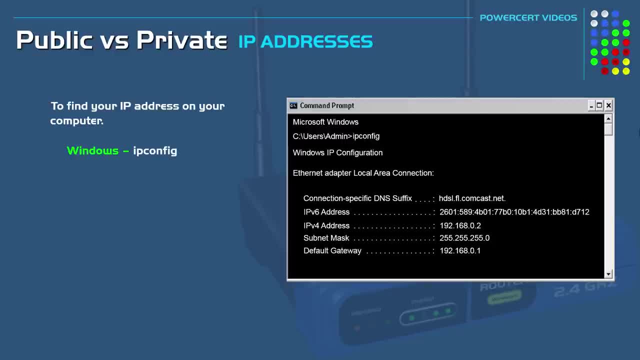 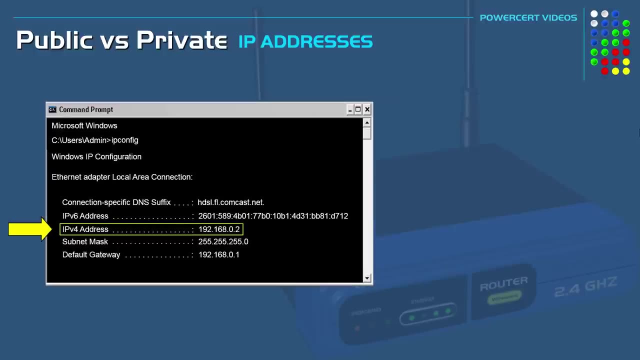 ipconfig. On Mac and Linux computers, you just open up a terminal and type ipconfig. So here is the IP address for this computer And, as you can see, this is a class C private IP address that has been given to us by our router. So, since this computer is assigned, 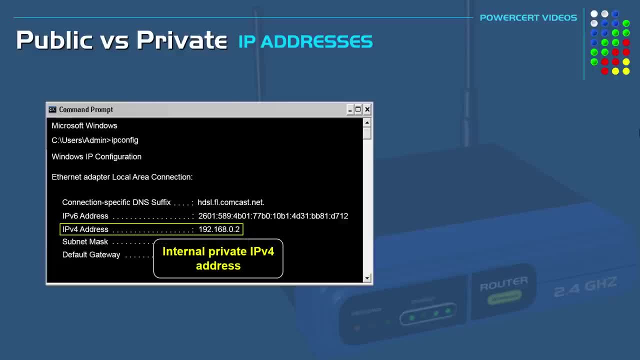 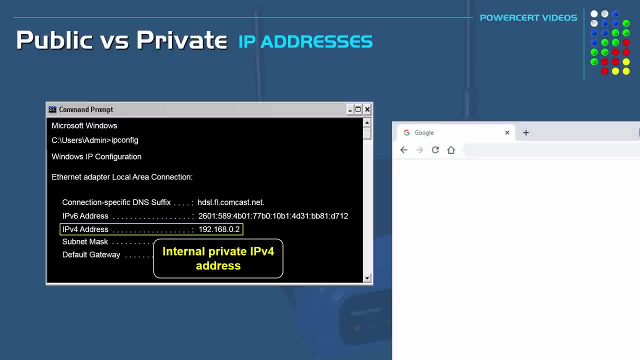 a private IP. it's not going to show our public IP. But if you want to know what your public IP address is, you just open up a web browser and then you will go to a website like whatsmyipaddresscom and that web page will show you your public IP address. 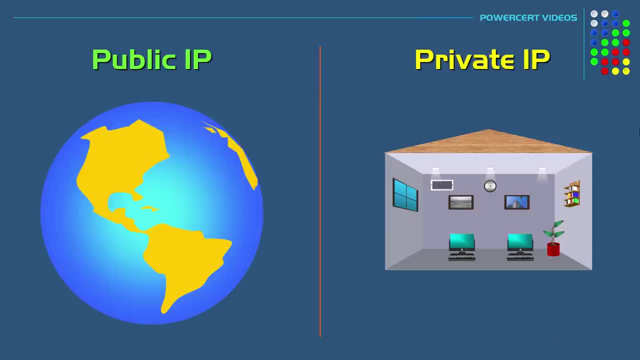 So, to summarize, public IP addresses are unique, while private IP addresses are non-unique, because the same private IP addresses can be used in other private networks. Public IPs are publicly registered, so they are able to access the internet, while private IPs are not publicly. 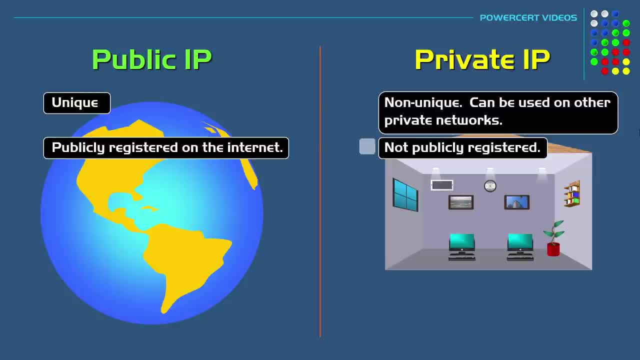 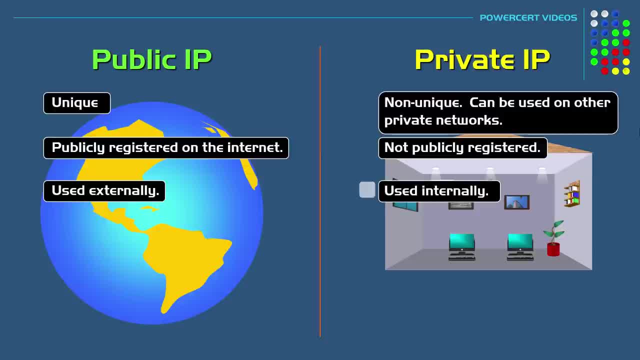 Private IPs are used internally on local networks. Public IPs are assigned by your internet service provider, while private IPs are assigned by your router. Public IPs are not free. you have to pay for them, but private IPs are free. And as far as security, public IPs are not secure because they 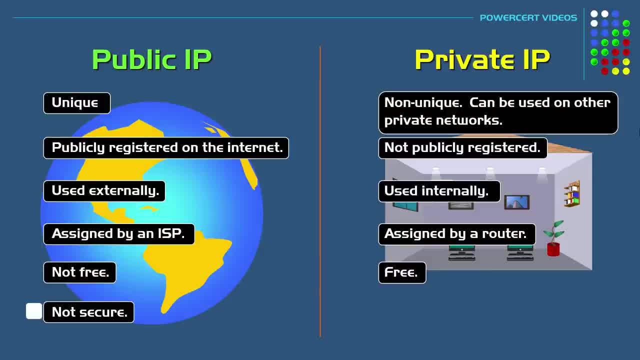 are used externally out on the internet, so they are traceable. So in order to make a public IP more secure, you have to add security to the internet. So in order to make a public IP more secure, you have to add security to the internet.